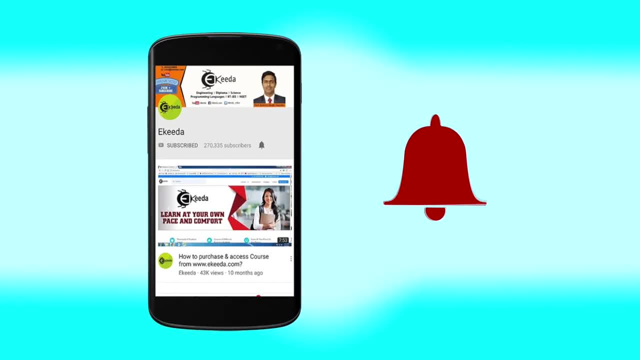 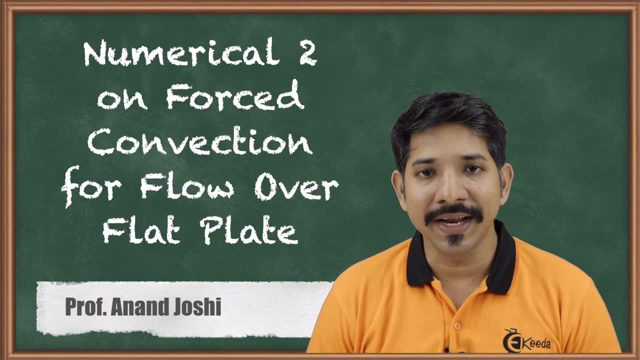 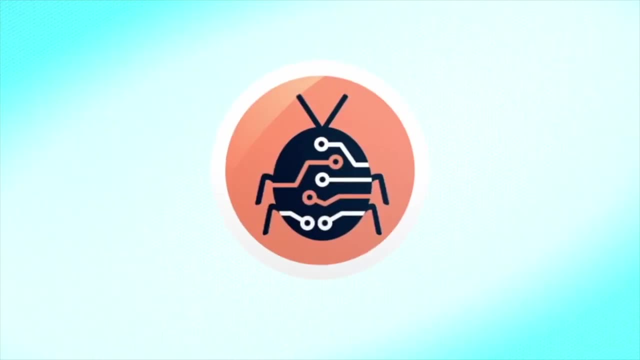 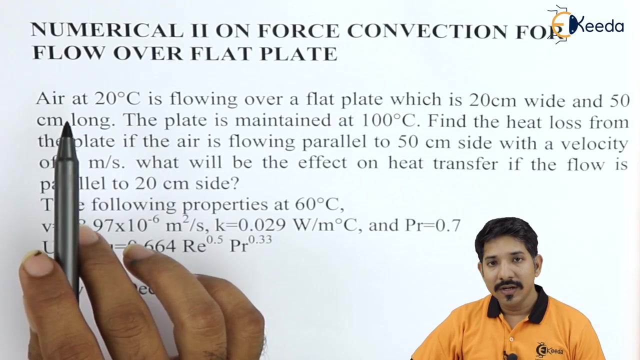 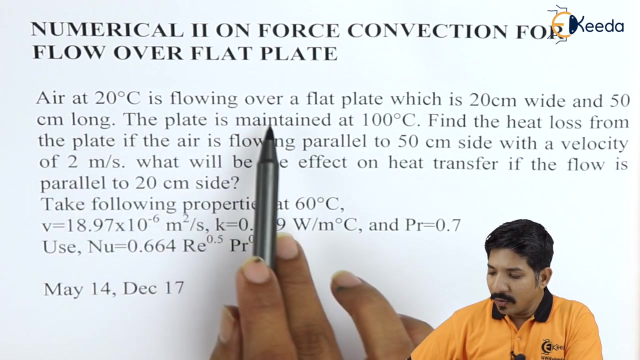 Hello friends, in case of an analysis of a force convection for a flow over a flat plate, the use of non-dimensionalist number is quite essential. Now let us look at the same with the help of one numerical. The numerical here says that air at 20 degree Celsius is flowing over a flat plate which 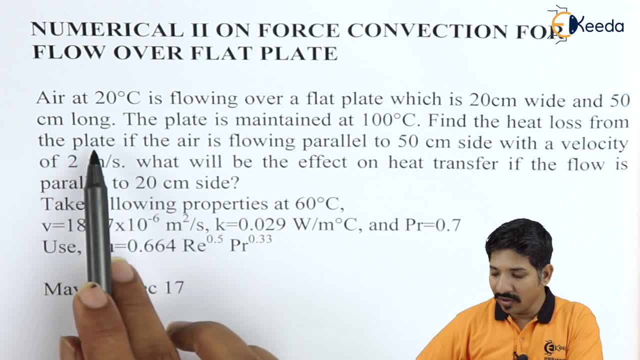 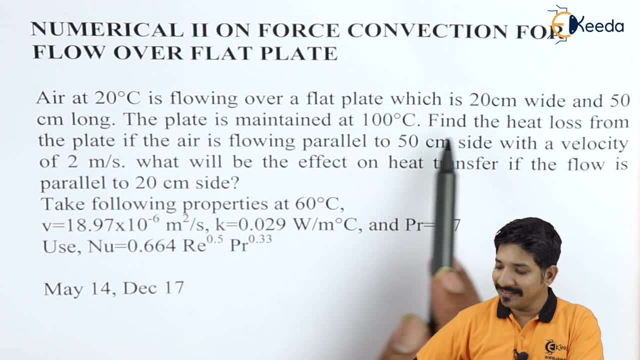 is 20 centimeter wide and 50 centimeter long, So they have given the air temperature and in the dimensions of the plate. The plate is maintained at 100 degree Celsius. Find the heat loss from the plate in the plate If the air is flowing parallel to the 50 centimeter side with the velocity of 2 meter per second. 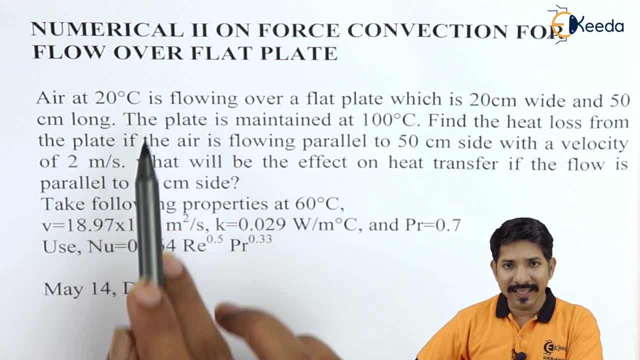 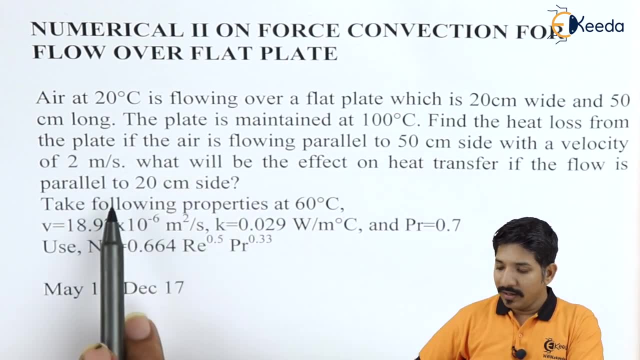 So they have given us the velocity of the air and the temperature of the air, and then they have given us that the air flow is parallel to the 50 centimeter side. In the second case they are saying: what will be the effect on the heat transfer if the 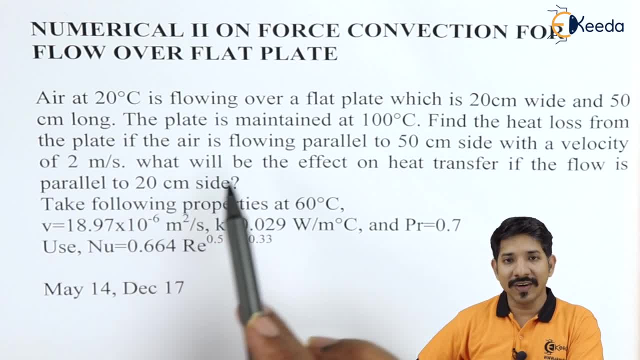 flow is parallel to 20 centimeter side. So in the first case the air flow is parallel to 50 centimeter side and in the second case the air flow is parallel to the 20 centimeter size. they have given us that the property at 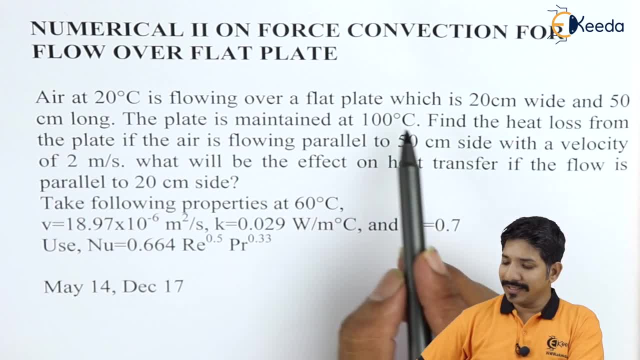 60 degree Celsius. that is the mean temperature. the temperature that they have given is 120, so the mean temperature is 60. so at 60 degrees Celsius they have given us the various thermophysical properties, such as: kinematic viscosity is given as 18.97 into minus 6 meter square. second. 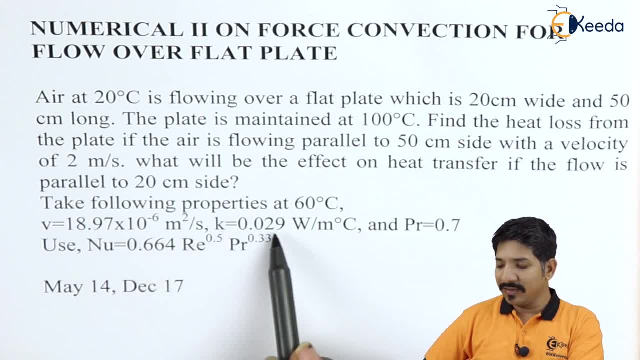 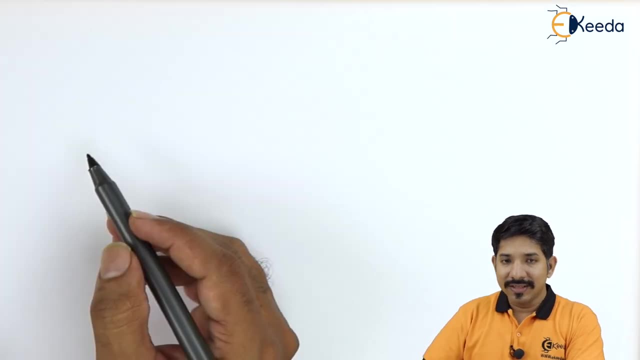 then they have given us the thermal conductivity as 0.029 watt per meter degree Celsius, bundle number is given as 0.7 and they have given us a co-relationship. this question was asked in May 14 and December 17 in case of a Mumbai University. now let us start solving this question. so 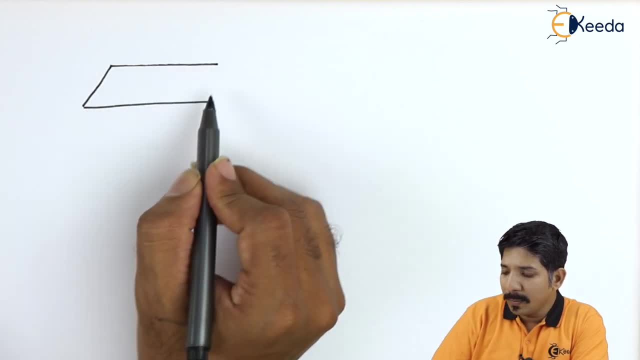 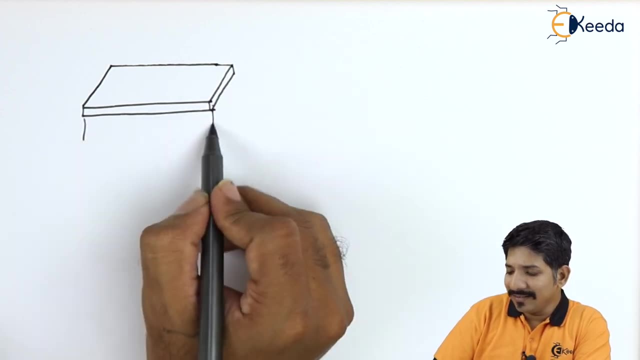 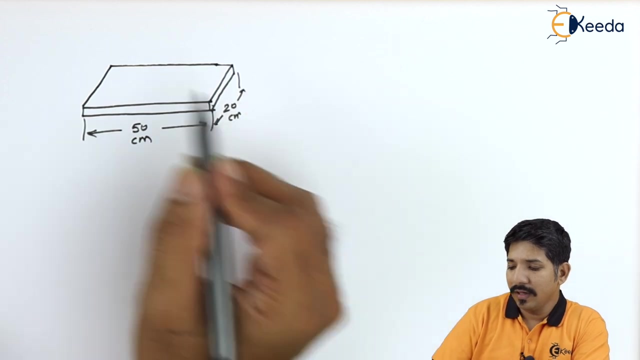 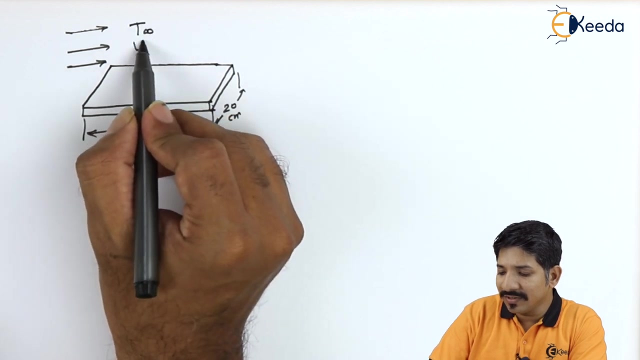 they have given us a plate whose thickness is unknown, so we will keep the thickness as it is. they have given the this as 50 centimeter and this as 20 centimeter. on this we have a air flow. for the air flow, the temperature is, let's say t, infinity velocity, let's say u. similarly, the surface temperature is: 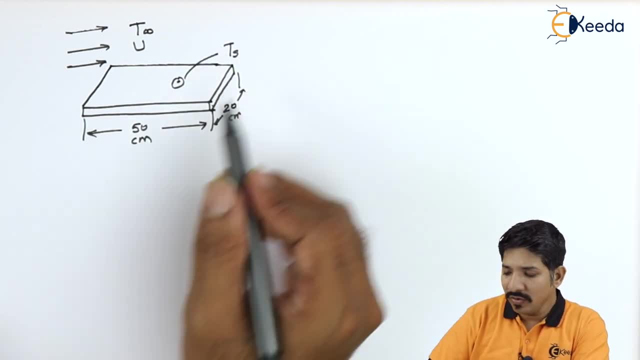 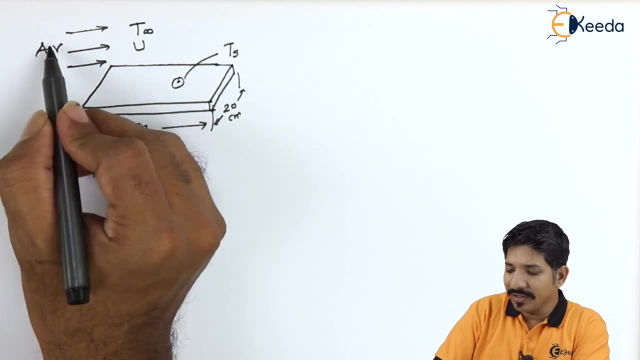 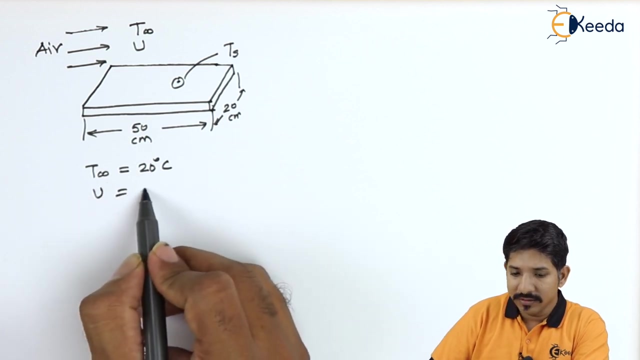 let's say ts. now let us write down the things that we know in this. they have given the t infinity. that is the fluid temperature. the fluid in this case is air. obviously the air temperature that they have given is 20 degrees Celsius, then the velocity is: 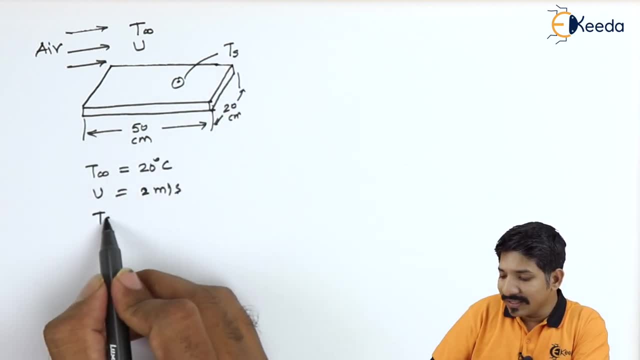 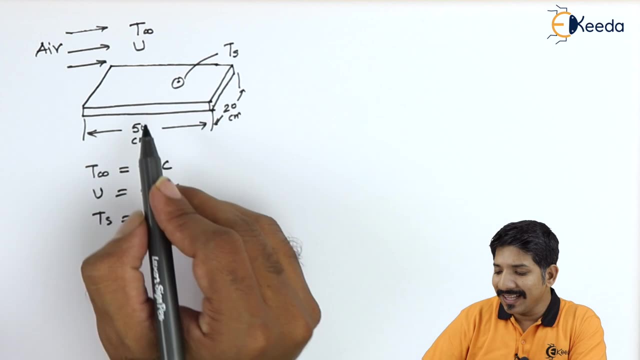 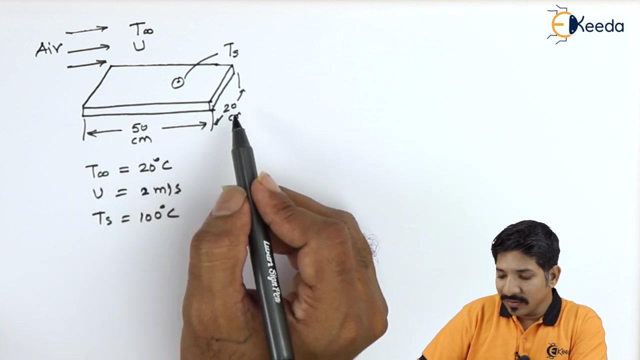 2 meter per second. the surface temperature is 100 degrees Celsius. now, these are the given things. now, along with that, they have given us the dimensions of plate which we have drawn over here. now, what they are asking us to find out? they are asking to find out in the first. 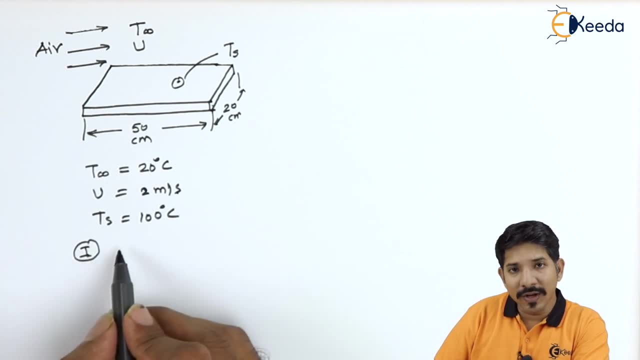 case, If the flow is parallel to 50 mm side, then what is the value of Q dash? So let me write Q dash 50. and in the second case, what is the value of Q dash if the air flow is parallel to 20 centimeter side? 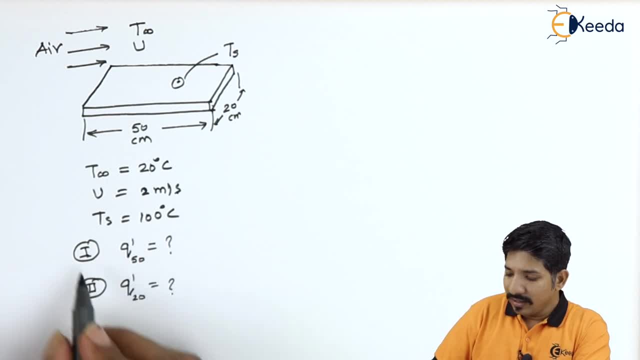 So let us write this as Q dash 20.. Now, these are the two things that they are asking us to find out. and then they have given us various thermophysical properties at mean temperature that is, 60 degree Celsius. I have not mentioned it here. 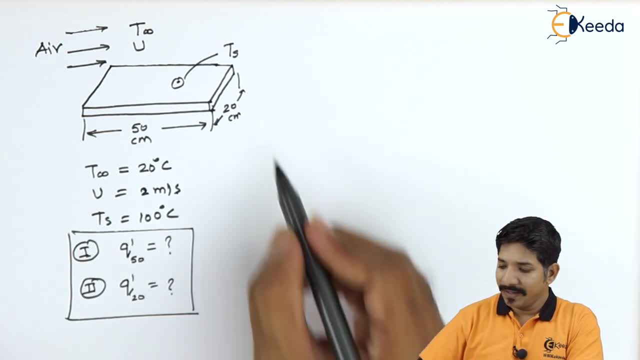 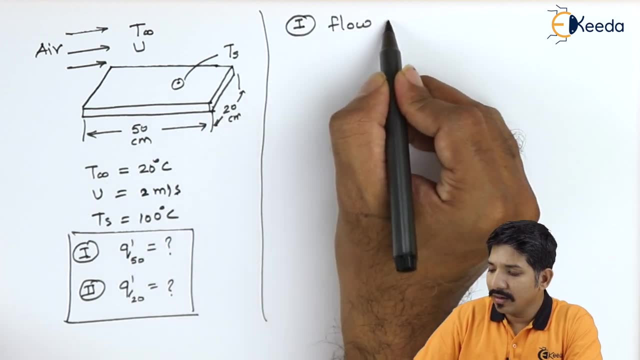 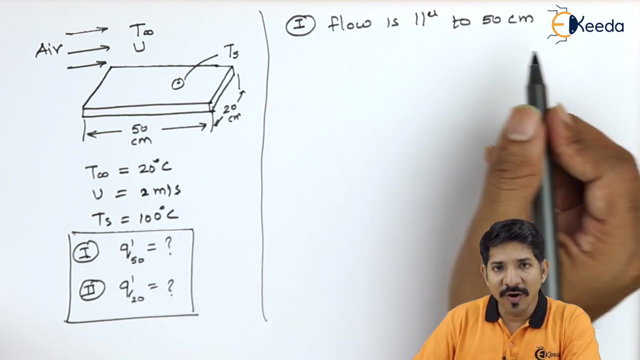 So we are obviously going to use it in the calculation itself. Now let us go for the solution. Now. I am taking the first case when the flow is parallel to 50 centimeter side. Now how to go about this? The first thing that we need to know is finding the Reynolds number. 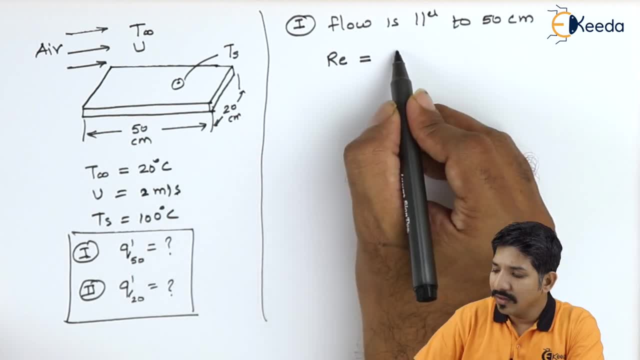 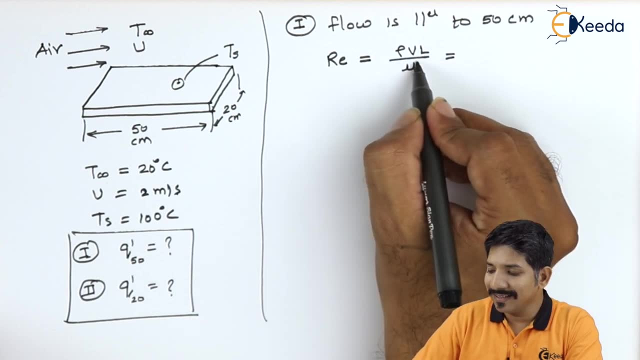 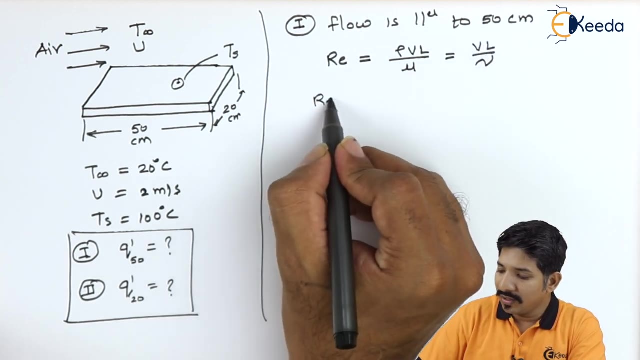 The Reynolds number in this case is given. It is given as rho VL upon mu. Now again, in this case the dynamic viscosity is not given, So we will write this as VL upon mu. So the Reynolds number that we are going to get is: the velocity is 2 meter per second. 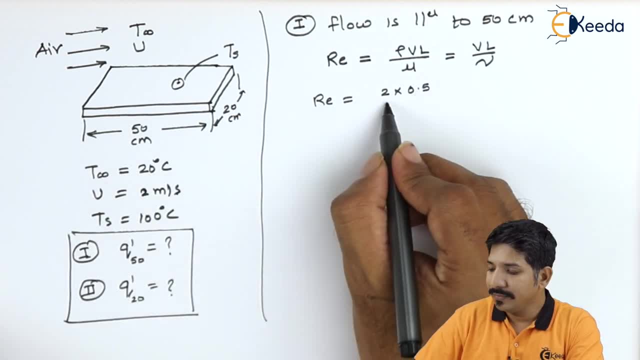 The length here is 50 centimeter, So that is 0.5 meter, And the kinematic viscosity that they are given is 50 centimeter. So that is 0.5 meter And the kinematic viscosity that they are given is 50 centimeter. 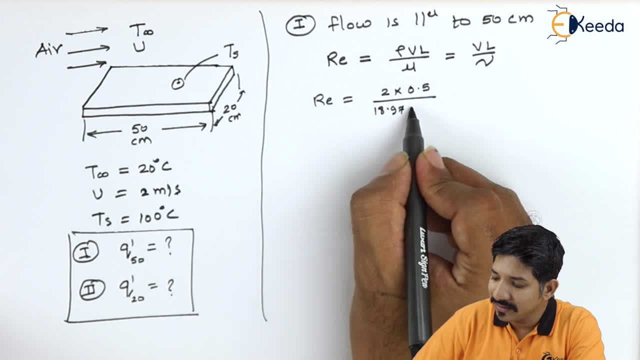 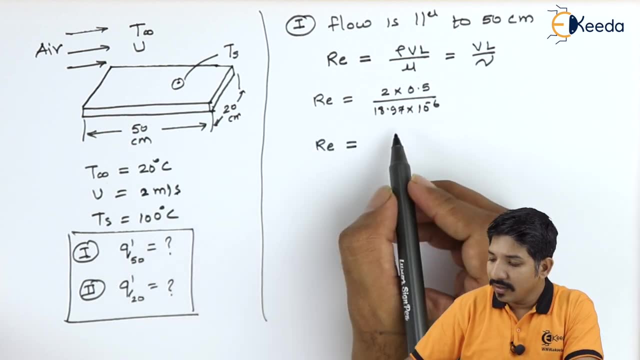 So that is 0.5 meter. So that is 0.5 meter And the kinematic viscosity that they are given is 0.7 meter, which is 18.97 into 10 raised to minus 6.. Now again, if I solve this, I will get some Reynolds number. 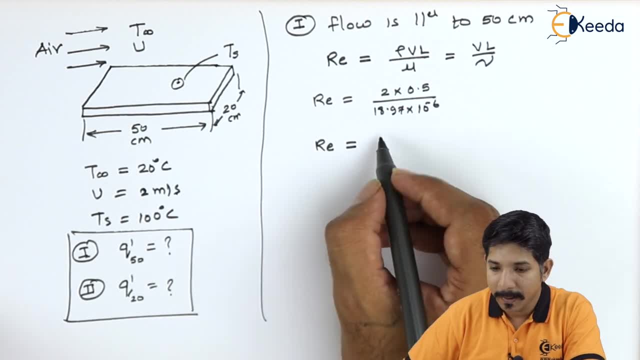 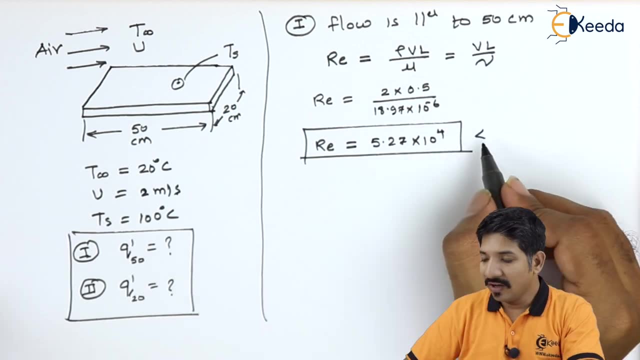 So the Reynolds number that we are getting at the end of this solution is 5.27 into 10 raised to 4.. Now, here now we can say that since it is less than 3 into 10 raised to 5, the flow must be: 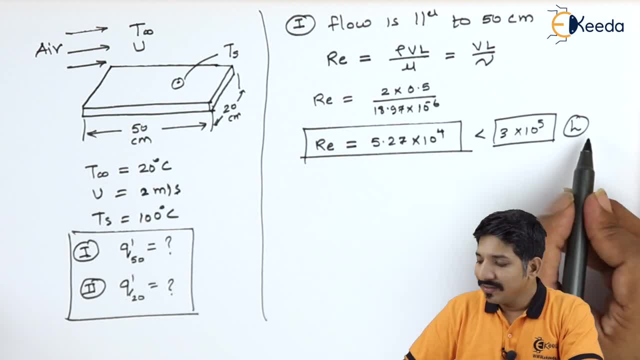 a laminar flow. See, we know that for the serial per unit or for the total per unit per unit, we are going to give a laminar flow. Let us say we have a laminar flow. So let us say we have a laminar flow. 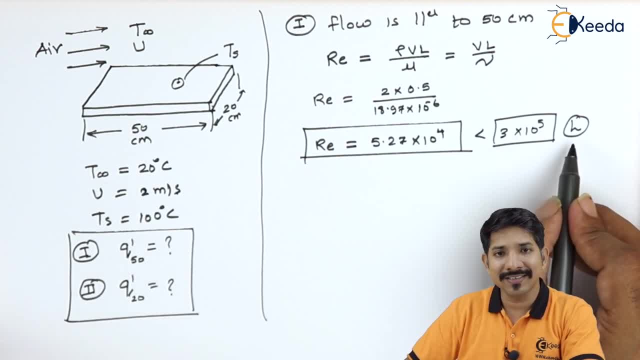 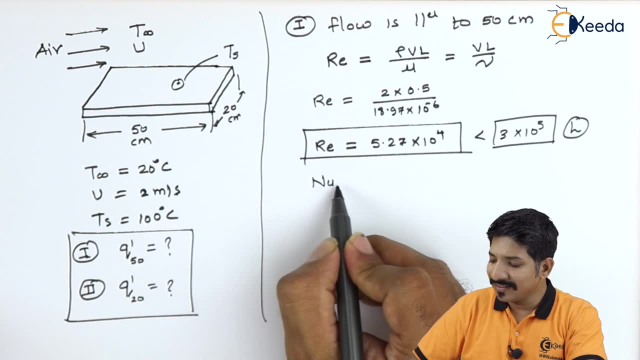 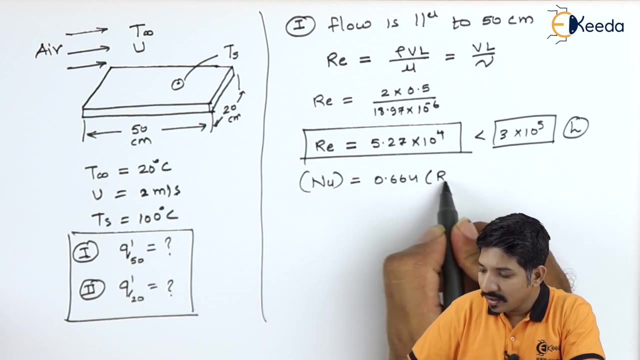 see, we don't really require this thing, because in this case they did not ask us to find if the flow is a laminar or turbulent. they have simply given us a relationship of Nusselt number, which is NU, equal to 0.664, Reynolds number is to 1 by 2 and Prandtl number is 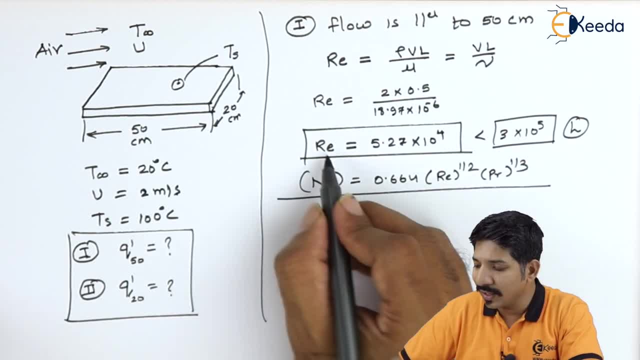 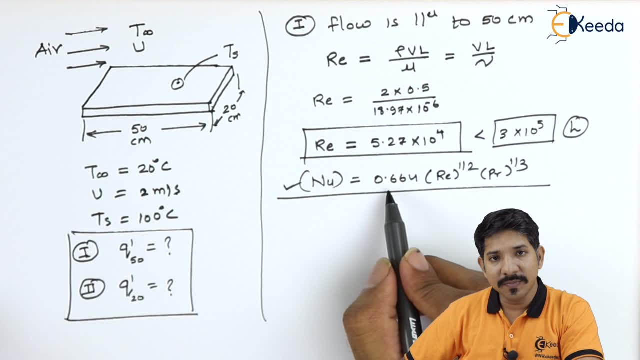 to 1 by 3.. So what we are going to do? we are going to simply substitute the Reynolds number in this equation, and the Prandtl number is given as 0.7 itself the Nusselt number is given- it is 0.664- into Reynolds number is to 1 by 2 and Prandtl number is to 1 by 3.. 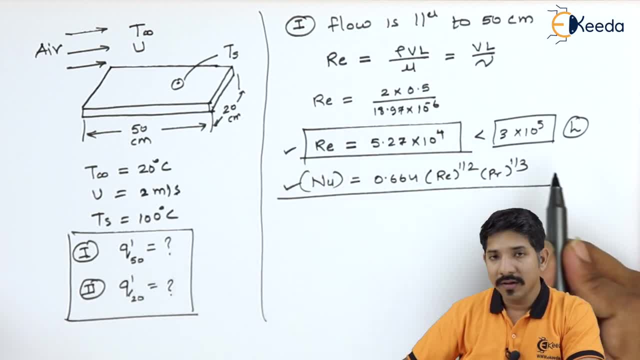 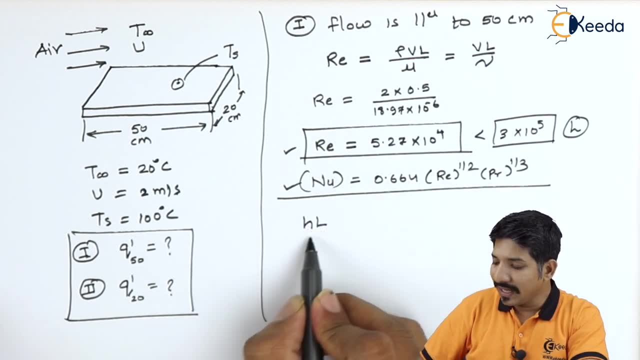 Now this thing is already given to us. we have already found the Reynolds number, So let us put the numbers over here. What is the Nusselt number? it is given as H, L upon K. In this case, we don't know the value of H. that is what we are going to find it out is. 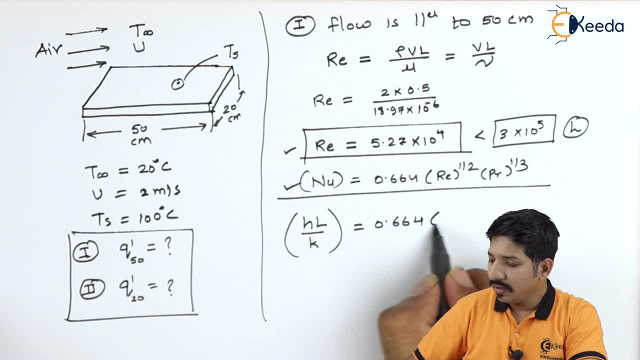 equal to 0.664 Reynolds number. Reynolds number is to 1 by 2. Prandtl number is to 1 by 3.. So now the length here is, in this case they have given us. in the first case the flow is parallel to 50 centimeter. 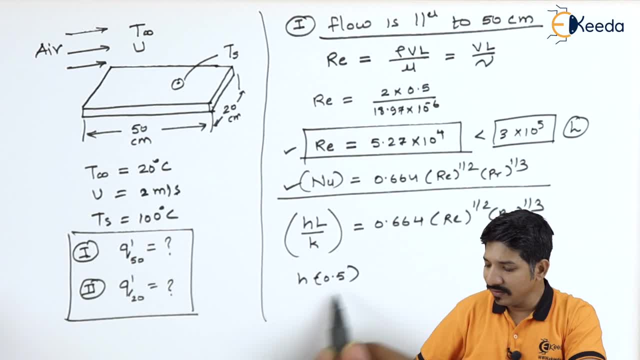 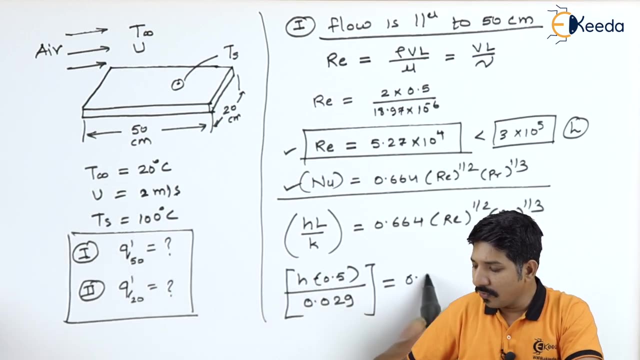 side. so my length is obviously 0.5. the thermal conductivity is given. it is given as 0.029 is equal to 0.664 Reynolds number. So what we are going to do now, we are going to find the Reynolds number, So we have the. 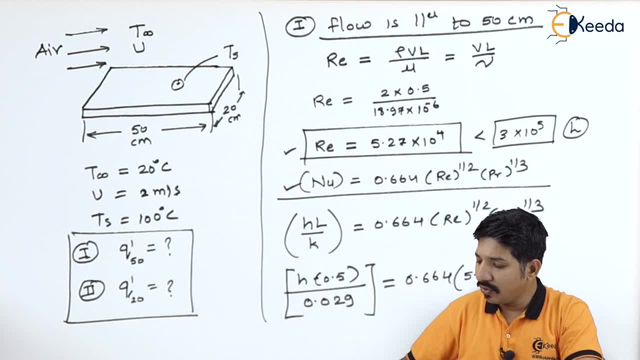 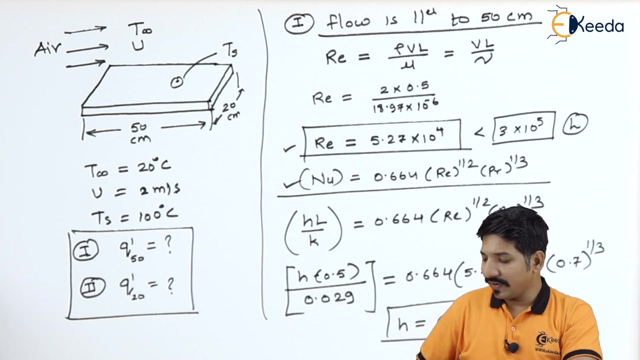 the number is 5.27 into 10. raise to 4, and the Prandtl number that they have given is 0.7. raise to 1 by 3.. Now, again, in this entire equation, the only unknown that we need to solve is H. The value of H that we are getting is 6.775 Watt per meter square degree Celsius. 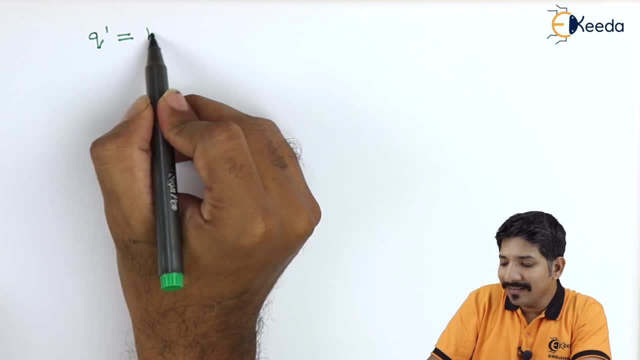 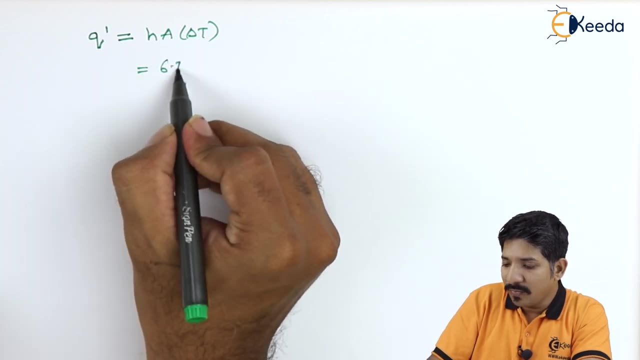 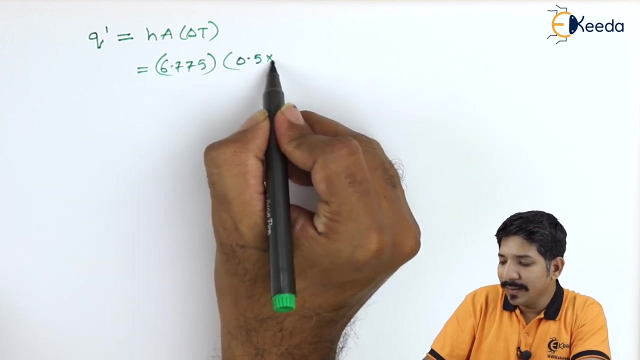 By Newton's law of cooling, the Q dash can be written as H A, Delta, T. Now here, the value of H that we have got is 6.775.. The area in this case is 0.5 multiplied by 0.2, since they 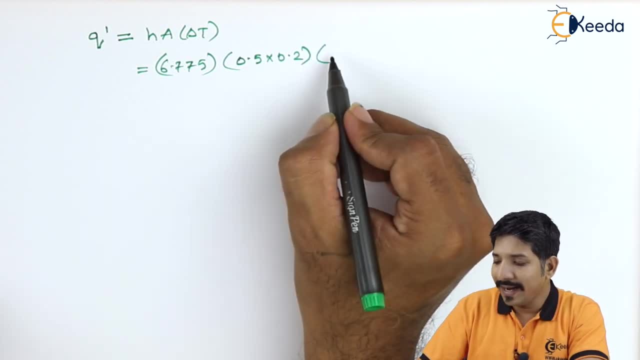 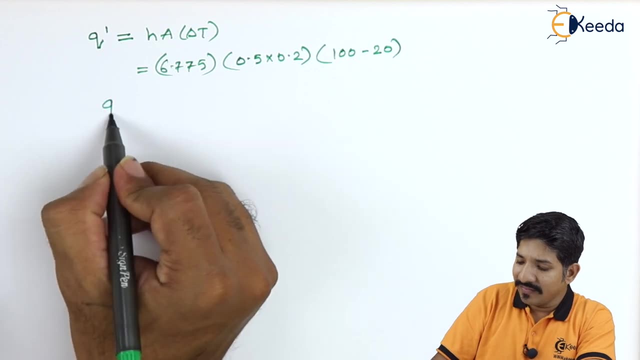 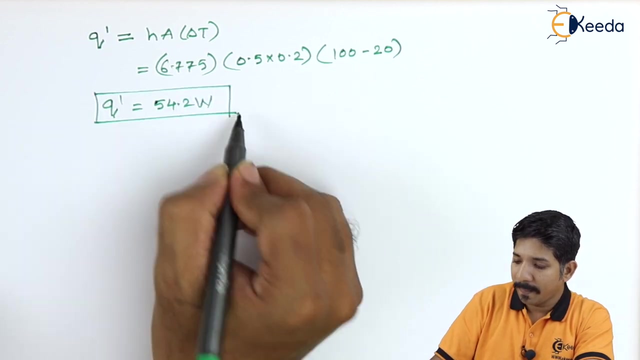 have given the dimensions as 50 centimeter by 20 centimeter and the temperature is. they have given the surface temperature as 100 and the air temperature is 20.. So with this again we can find out the value of H. In this case the value of Q dash we are getting is 54.2 Watt. This was the first case In the 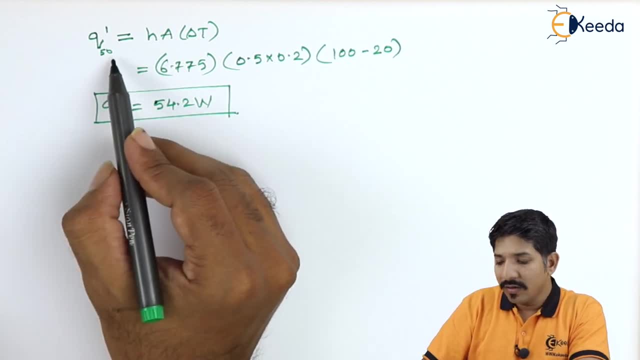 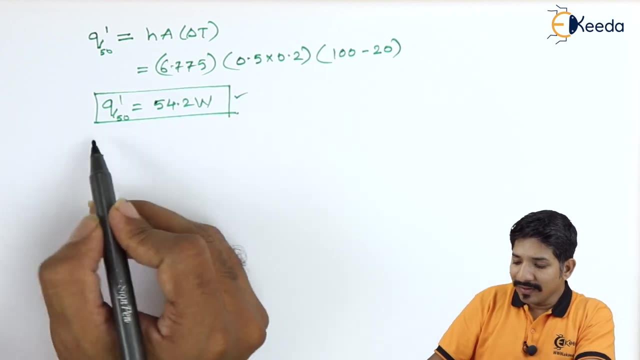 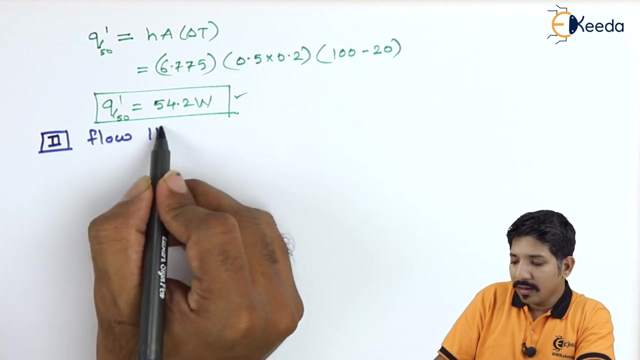 first case, the heat transfer rate that we have found was when the flow is parallel to the 50 centimeter side. So that is why we have written this Q dash of 50.. Now let us go for the second case. So in the second case my flow is parallel to: 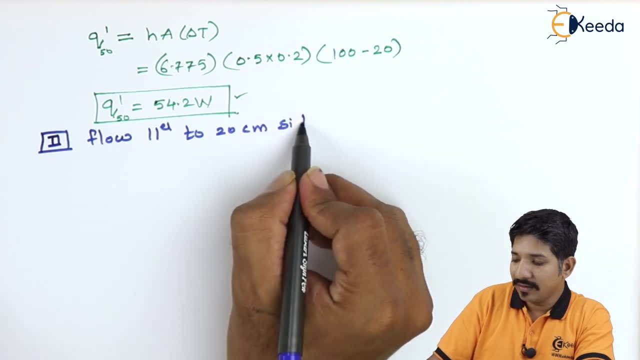 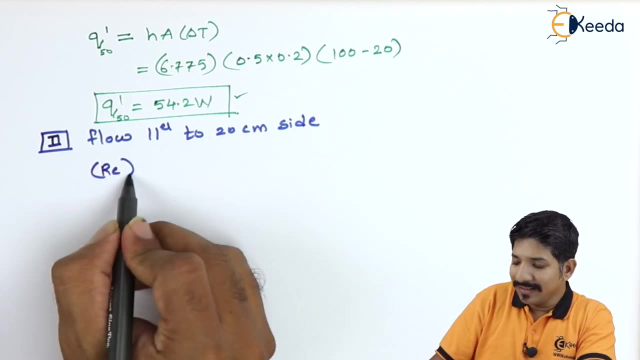 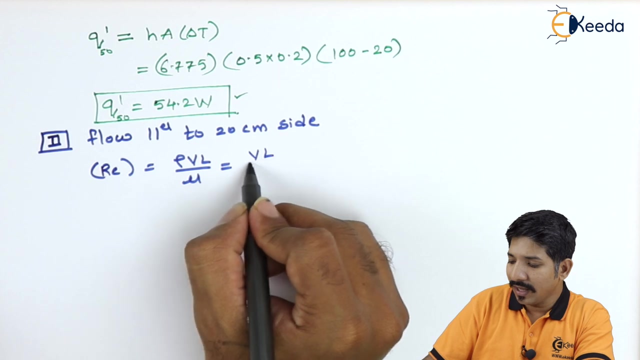 the 50 centimeter side, which is going to be 25 H at theıp 20 centimeter. 20 centimeter side. If that is the case, then again we will Weber to figure it out: the Reginald number: What's the amount number? it is again given as Rho. 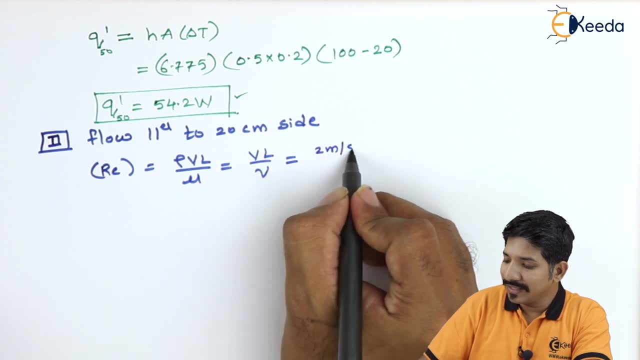 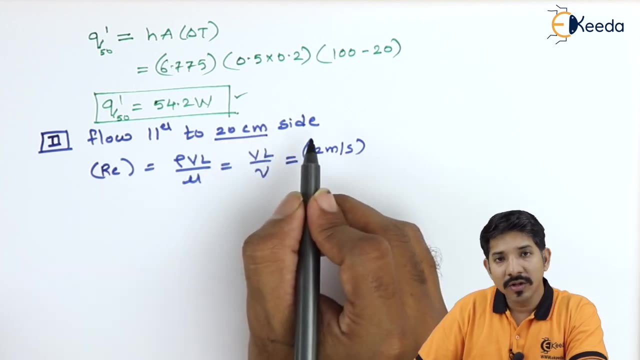 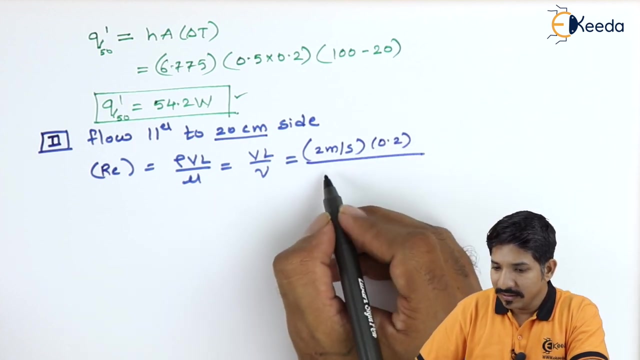 V L upon nu. We can modify this by writing V L upon nu. The velocity in this case is the one that is parallel to flow. So that is 20 centimeter. So it becomes 0.2 and the kinematic viscosity in this case is given as 18.97 into 10 raise to minus 6.. So if I 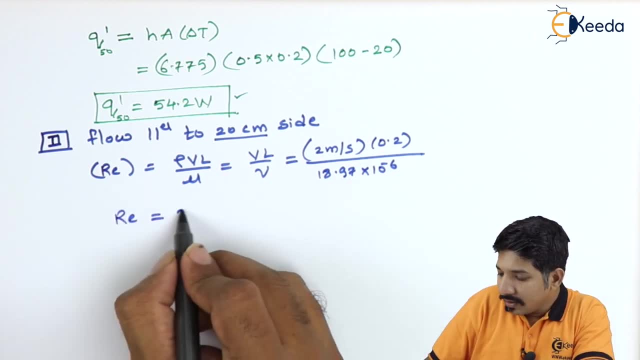 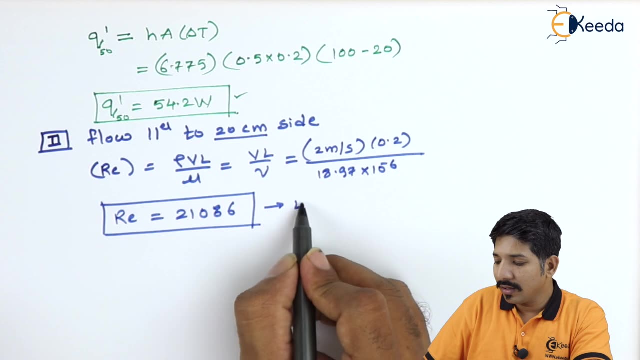 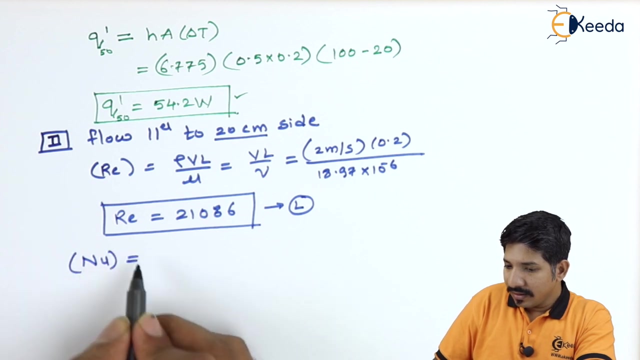 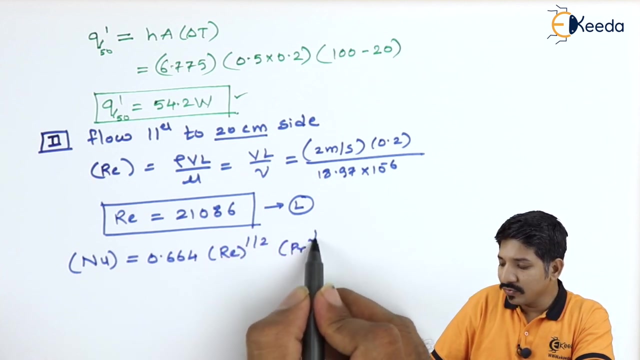 solve this. I will get the Reynolds number as 21086.. So again we can write that this also is a laminar flow. Now let us use the corollary shift. Nusselt number is given as 0.664, Reynolds number raise to 1 by 2 and Prandtl number raise to 1 by 3.. Nusselt number: 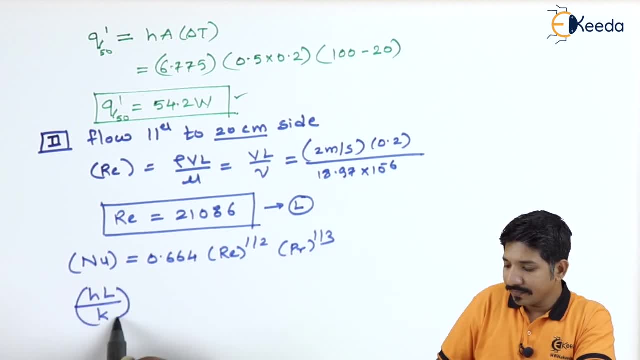 is again given as HL by K. Now, in this case, the value of L is 0.2 and the value of K is again 0.2.. They were given these two numbers, so the only unknown should be the value of H. So let us. 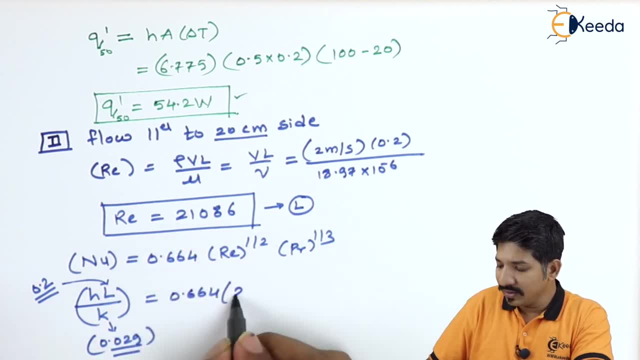 put that 0.664, the reynold number is 21086. raise to 1 by 2. reynold number is 0.7. raise to 1 by 3.. So if I solve this, the value of H- that we are getting 10.7 watt per meter square. 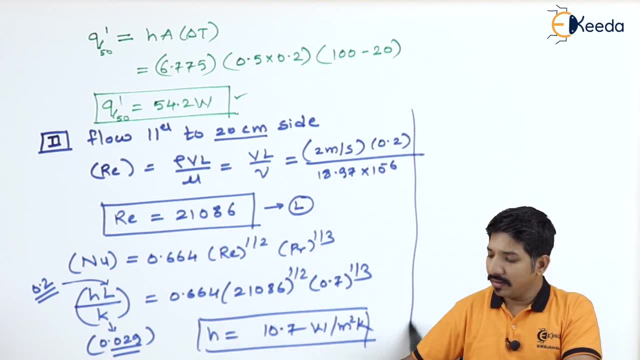 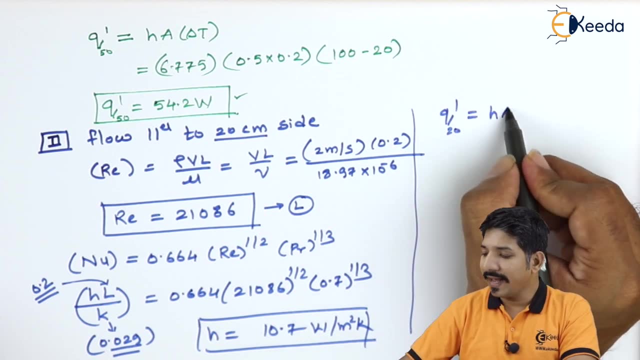 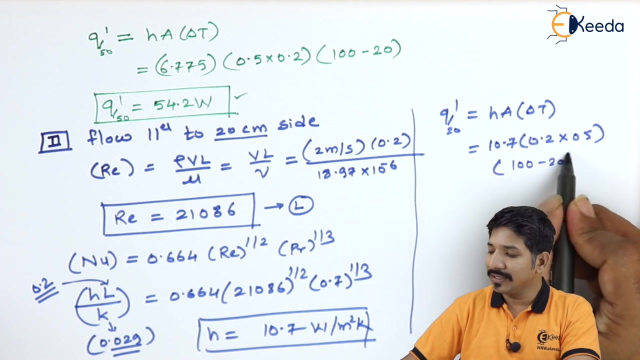 Now again, we know that the heat transfer coefficient is given by Newton's law of cooling as H A delta T. So the value of H is 10.7, the area will be again 0.2 multiplied by 0.5 and the temperature difference is again 100 minus 20. the 100 is a surface temperature, 20 is 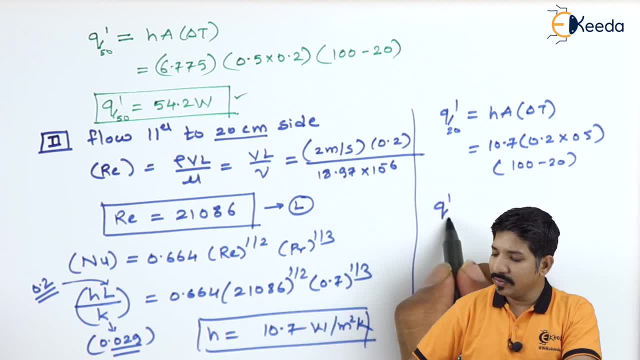 the air temperature difference. So from this, The value of Q dash by 20 that we are getting is 85.7.. So what can we conclude? we can conclude that Q dash by 20 we are getting is higher than Q dash by 50..